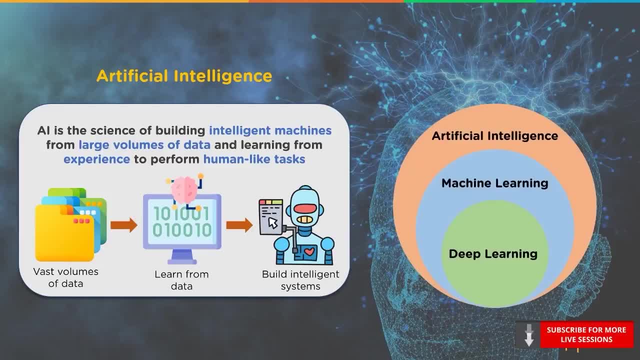 machine learning are the two subsets of artificial intelligence, So you need both machine learning algorithms and deep learning networks to build intelligent systems. AI is now being widely used in almost every sector of business, such as transportation, healthcare, banking, retail, entertainment and e-commerce. 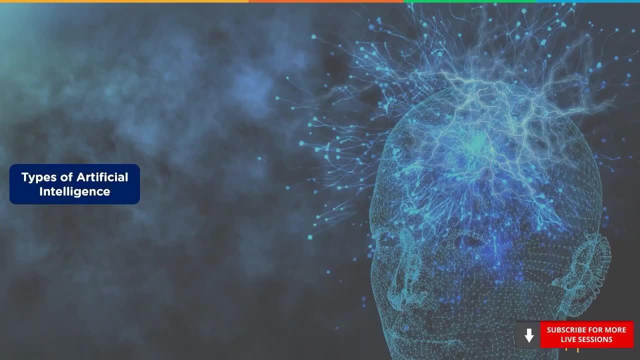 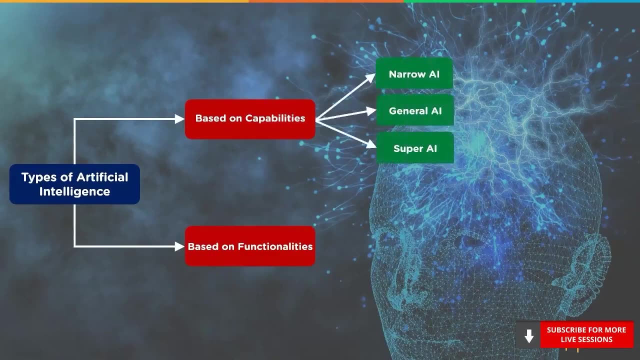 Now let's look at the different types of artificial intelligence. So AI can be classified based on capabilities and functionalities. Under capabilities, there are three types of artificial intelligence. They are Narrow AI, General AI and Super AI. Under functionalities, we have four types of artificial intelligence: Reactive machine, limited memory. theory of 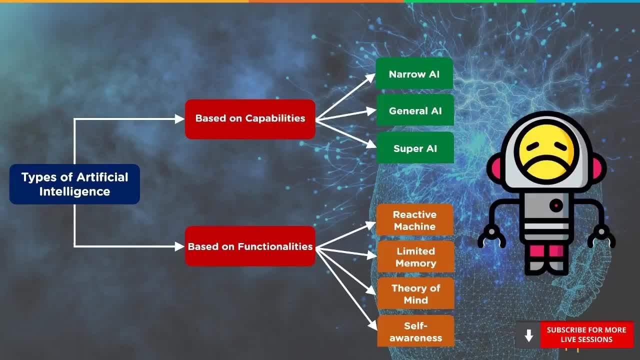 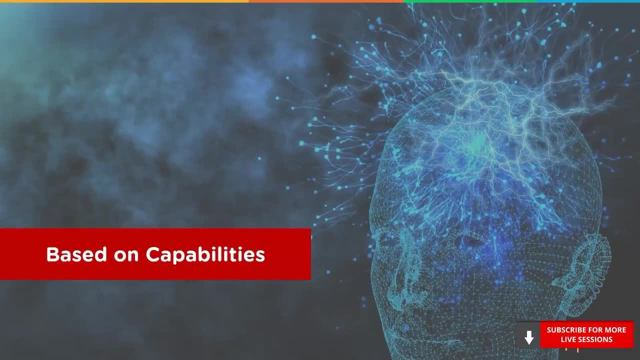 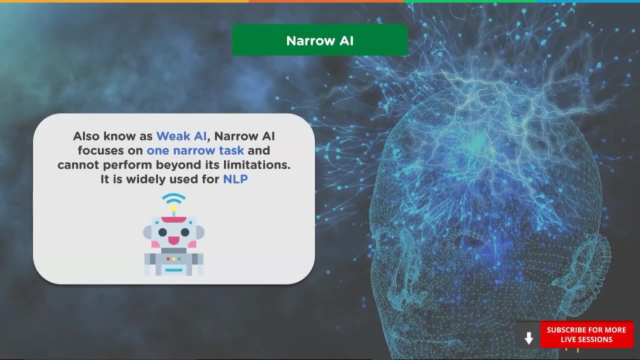 mind and self-awareness. Let's look at them one by one. First, we will look at the different types of artificial intelligence based on capabilities. So what is Narrow AI? Narrow AI, also known as Weak AI, focuses on one narrow task and cannot perform beyond its limitations. It aims at a single subset. 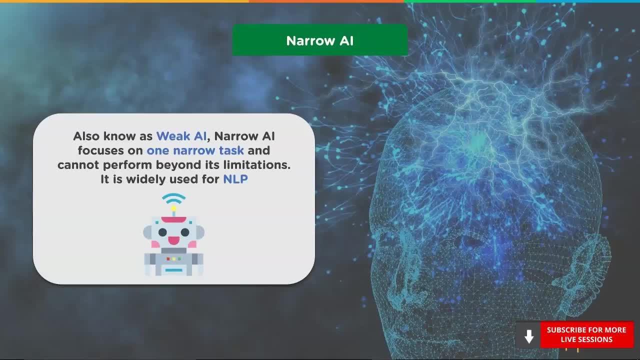 of cognitive abilities and advances in that spectrum. Applications of Narrow AI are becoming increasingly common in our day-to-day lives as machine learning and deep learning methods continue to evolve. Apple's Siri is a simple example of a Narrow AI that operates with a limited predefined 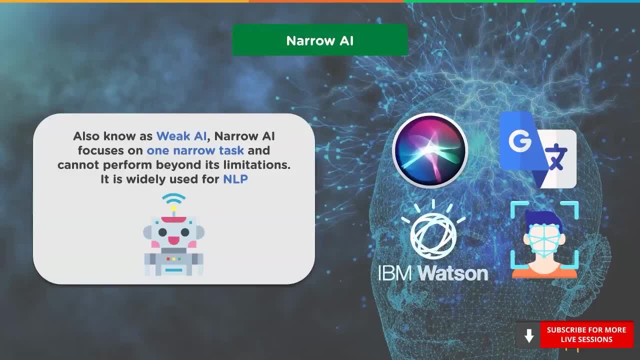 range of functions, Siri often has challenges with tasks outside its range of abilities. IBM Watson Supercomputer is another example of Narrow AI, which applies cognitive computing, learning and natural language processing to process information and answer your questions. IBM Watson once outperformed human contestant Ken Jenkins to become the champion on the 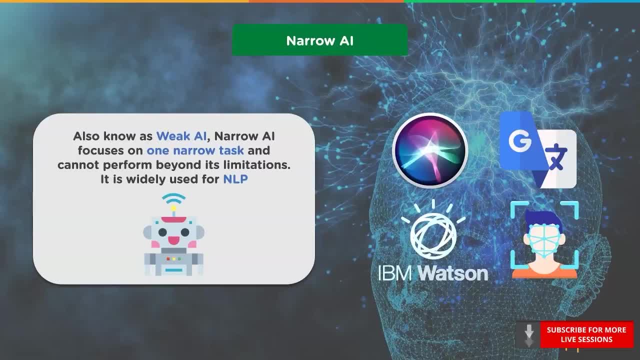 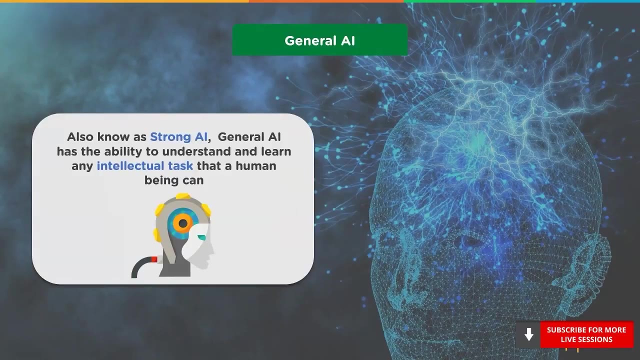 popular game show Jeopardy. Other examples of Narrow AI include Google Translate, image recognition software, recommendation systems, spam filtering and Google's Page Ranking algorithm. Next, we have General Artificial Intelligence, or General AI. General AI, also known as Weak AI, is an artificial intelligence based on the ability to process information and answer. 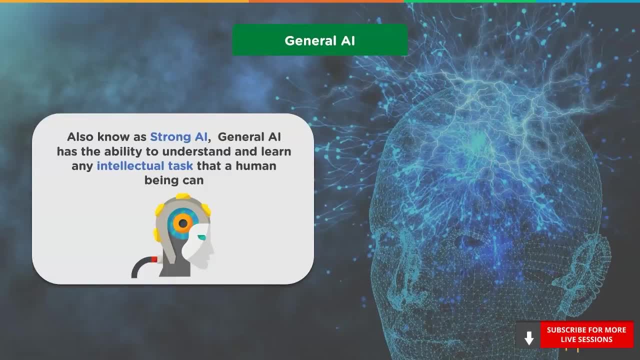 questions. It is the ability to understand and learn any intellectual task that a human can. General Artificial Intelligence has received a $1 billion investment from Microsoft through OpenAI. It allows a machine to apply knowledge and skills in different contexts. AI researchers and scientists have not achieved Strong AI so far. To succeed, they would need to find 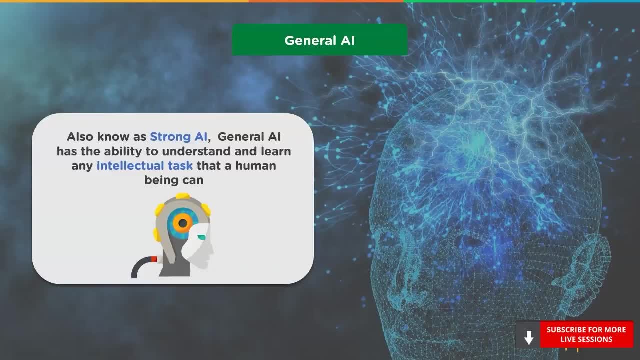 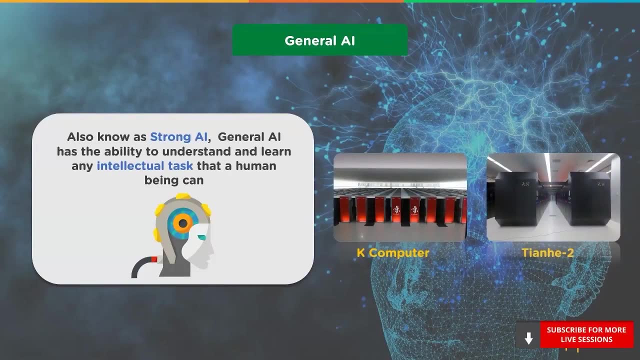 a way to make machines conscious, programming a full set of cognitive abilities- Fujitsu. Fujitsu built the K-computer, which is one of the fastest computers in the world. It is one of the most notable attempts at achieving Strong AI. It took 40 minutes to simulate. 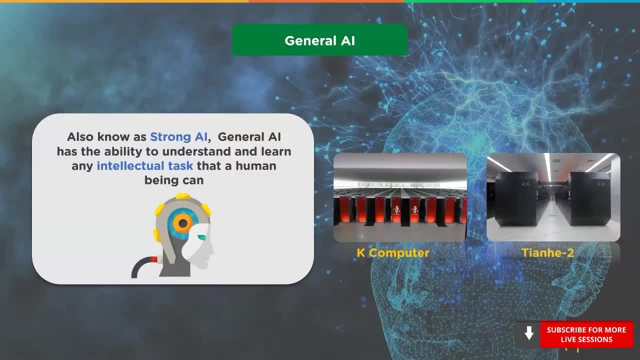 a single second of neural activity, so it is difficult to determine whether or not Strong AI will be achieved in the near future. Tianhe-2 is a supercomputer created by China's National University of Defense Technology. It currently holds the record for CPS at 33.86 petaflops. It is also considered the world's 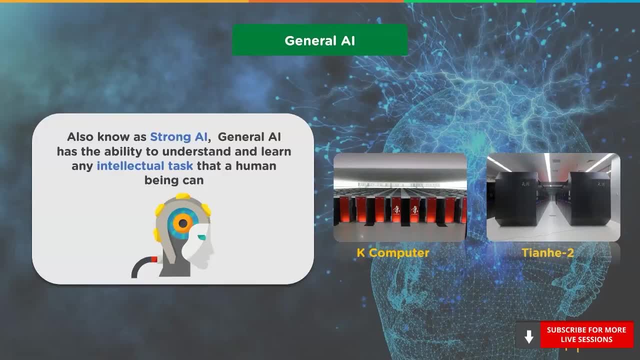 most advanced computer in technology, It is also one of the most powerful and powerful AI software in the world. We are working with Fujitsu to create a machine with stable and, although it sounds exciting, the human brain is estimated to be capable of one exaflop. 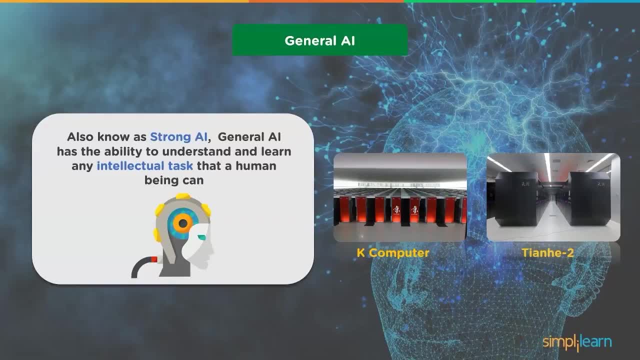 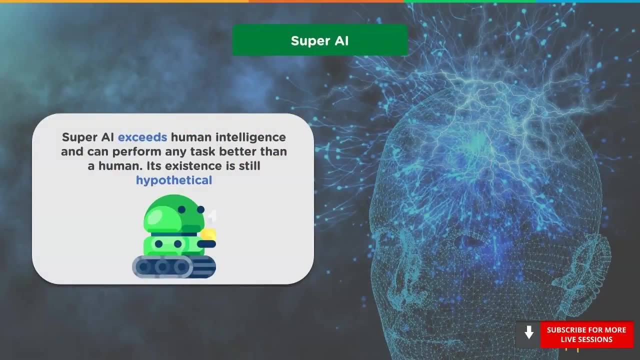 Now CPS means characters per second that a system can process. Third, in the list of AI that is based on capabilities, we have Super AI. Super AI exceeds human intelligence and can perform any task better than a human. The concept of artificial super intelligence sees AI evolved to be so akin to human emotions. 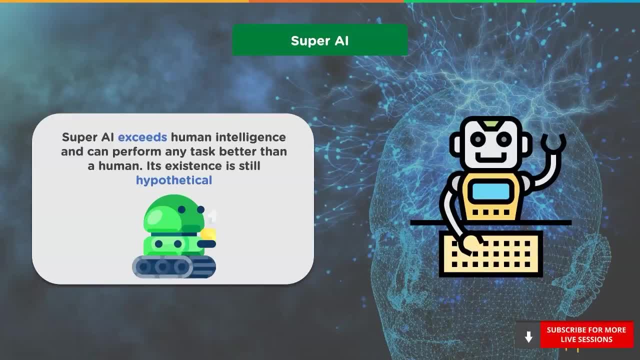 and experiences that it doesn't just understand them. It evokes emotions, needs, beliefs and desires of its own. Its existence is still hypothetical. Some of the key characteristics of Super AI include the ability to think, solve puzzles, make judgments and decisions on its own. 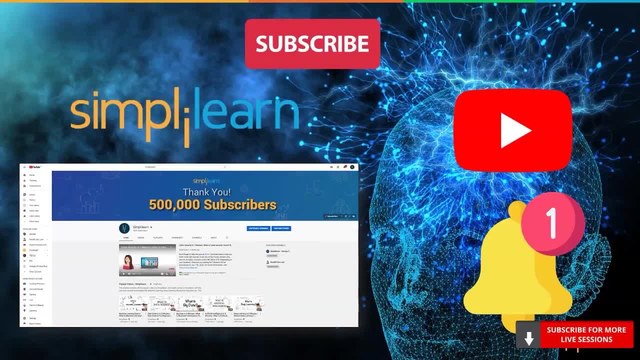 Now, if you have enjoyed watching this video so far, please make sure to subscribe to our YouTube channel and hit the bell icon to stay updated with all the latest technologies. Also, if you have any questions related to this video, please put it in the chat section. 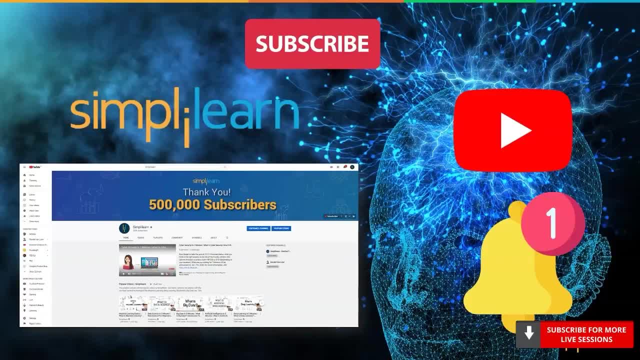 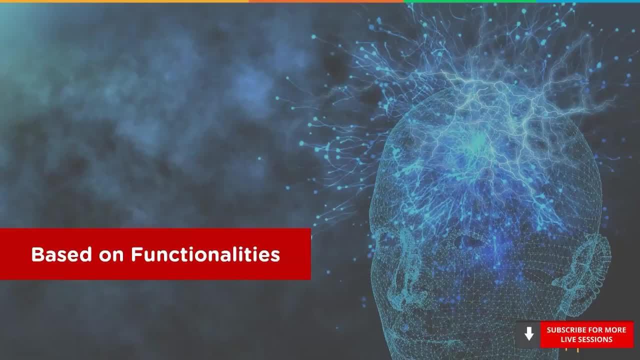 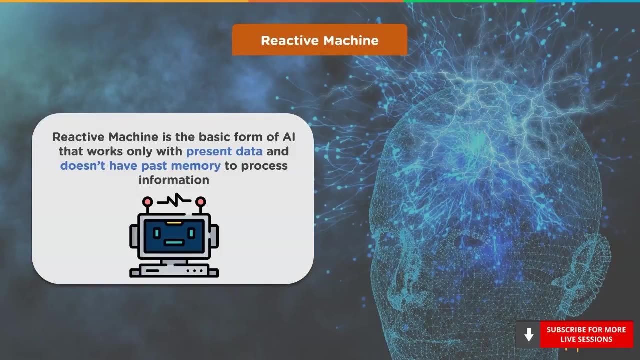 Our team of experts will help you address your questions. Moving ahead now, we will see the different types of artificial intelligence based on functionalities In this category. first, we have Reactive Machine. A reactive machine is the basic form of AI that does not store memories. 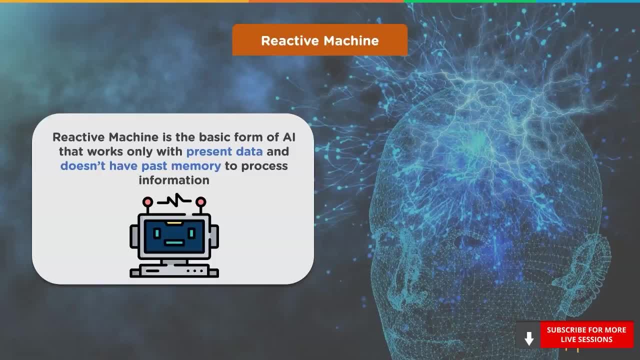 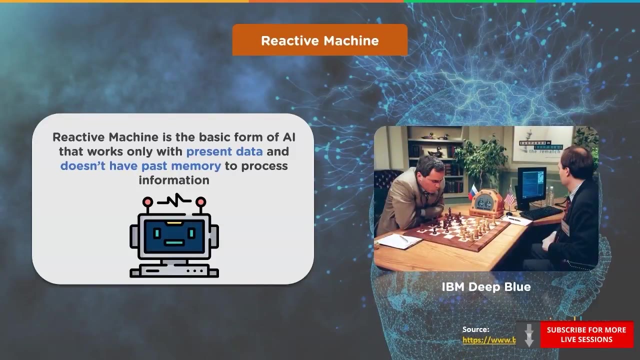 or use past experiences to determine future actions. It works only with present data. They simply perceive the world and react to it. Reactive machines are given certain tasks and don't have capabilities beyond those duties. IBM's Deep Blue, which defeated chess grandmaster Garry Kasparov. 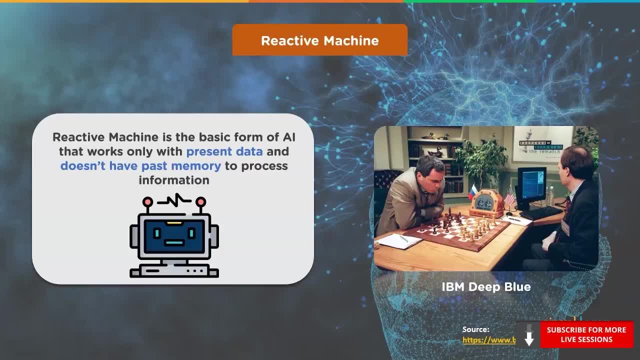 is a reactive machine that sees the pieces on a chessboard and reacts to them. It cannot refer to any of its prior experiences and cannot improve with practice. Deep Blue can identify the pieces on a chessboard and know how each moves. It can make predictions about what moves might be next for it and its opponent. 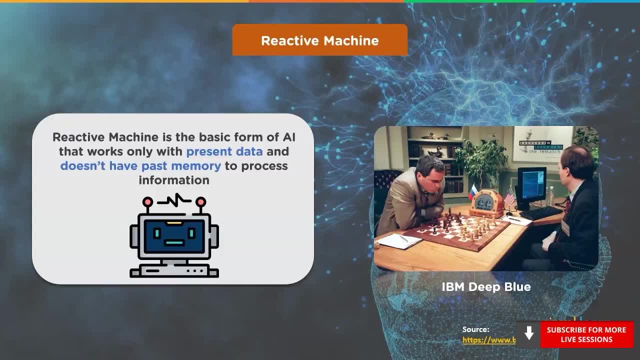 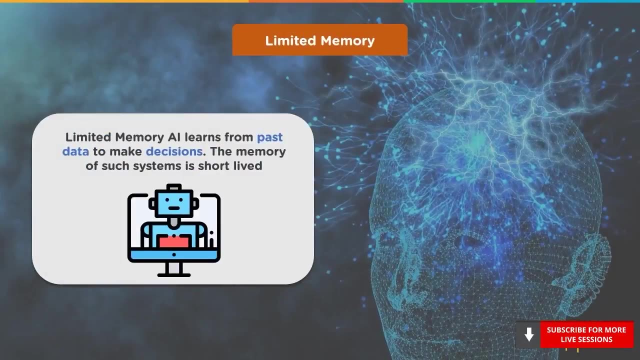 It can choose the most optimal moves from among the possibilities. Deep Blue ignores everything before the present moment. All it does is look at the pieces on the chessboard as it stands right now and choose from possible next moves Up. next we have Limited Memory. 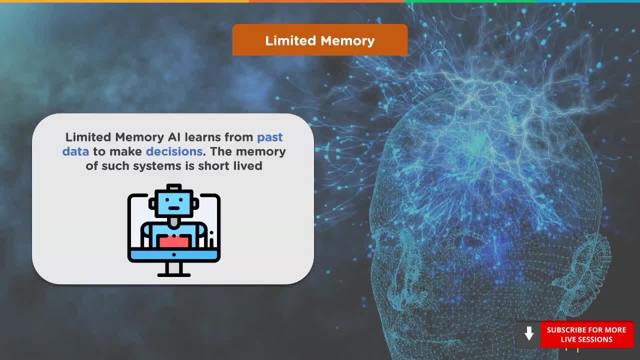 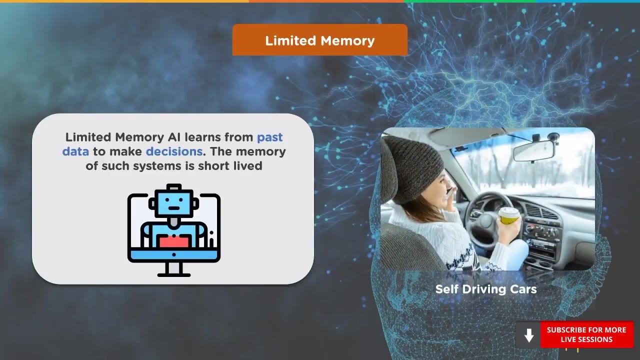 Limited Memory. AI learns from past data to make decisions. The memory of such systems is short-lived. While they can use this data for a specific period of time, they cannot add it to a library of their experiences. This kind of technology is used for self-driving vehicles. 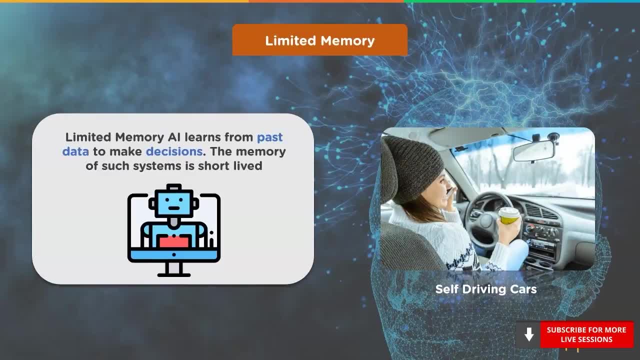 They observe how other vehicles are moving around them in the present and as time passes. That ongoing collected data gets added to the static data within the AI machine, such as lane markers and traffic lights. They are included when the vehicle decides to change lanes. 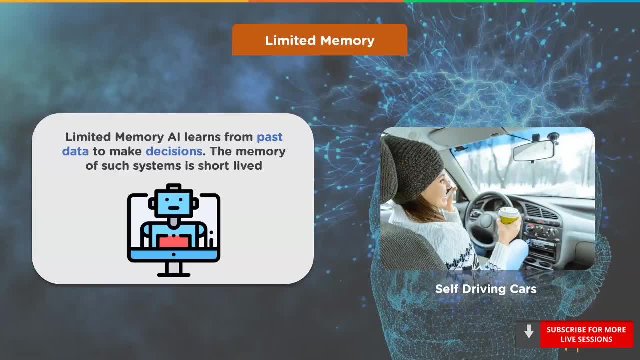 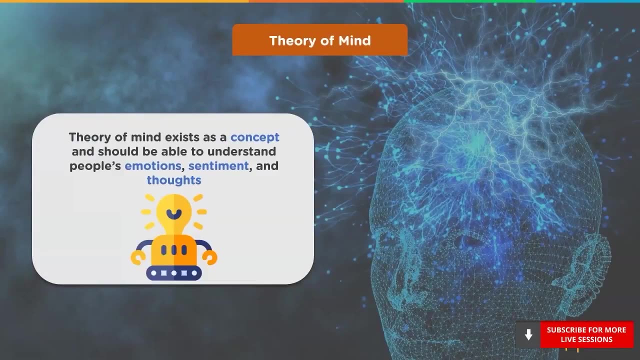 to avoid cutting off another driver or being hit by a nearby vehicle. Mitsubishi Electric is a company that has been figuring out how to improve such technology for applications like self-driving cars. Then we have Theory of Mind. Theory of Mind represents a very advanced class of technology. 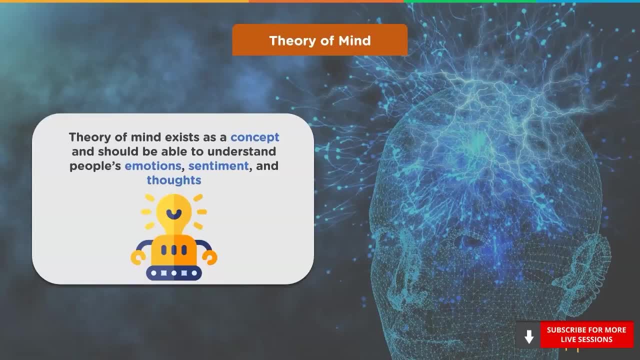 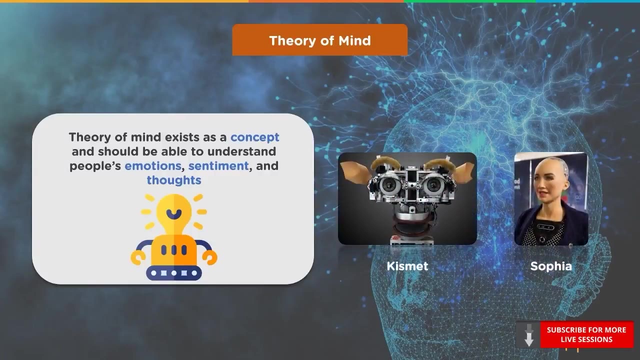 and exists as a concept. This kind of AI requires a thorough understanding that the people and the things within an environment can alter feelings and behaviors. It should be able to understand people's emotions, sentiment and thoughts, Even though a lot of improvements are there in this field,